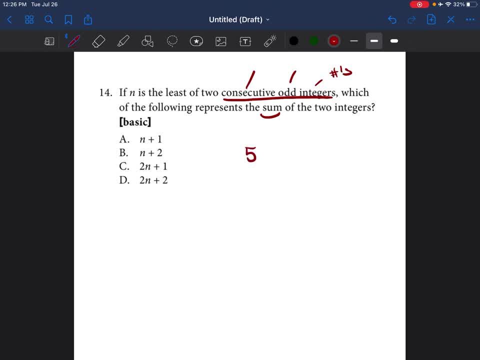 So they're just asking us, for example, if we had 5.. 7,, 9,, 11.. Those are all numbers or integers, They're all odd and they're all consecutive, coming one after another. Let's pretend for a second that 5 is n. 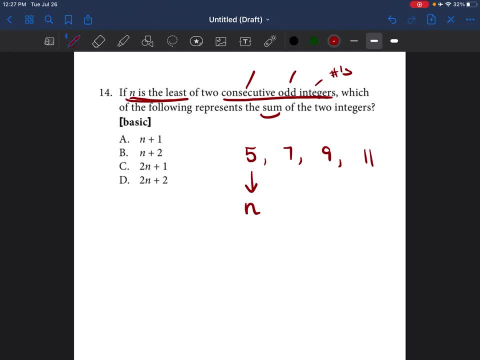 It says n is the least of the two numbers. Let's pretend that 5 represents n. In order to get from 5 to the next number in sequence, the next consecutive number, you have to add 2.. 5 plus 2 is 7.. 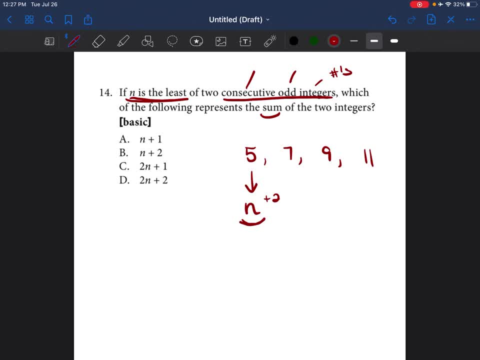 So in order to go from the first integer, n, to the next integer, you'd have to do n plus 2.. So the first integer is represented by n. The second integer would be n plus 2.. So they simply said: what is the sum of the two integers? 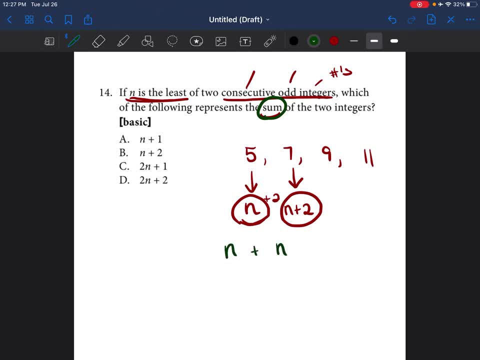 So you would just add n plus n plus 2.. So how do we add n plus n plus 2? I go ahead and put the invisible 1 in front of the two n's so that we can combine like terms. I know that these two terms are alike because they both have the same variable, n. 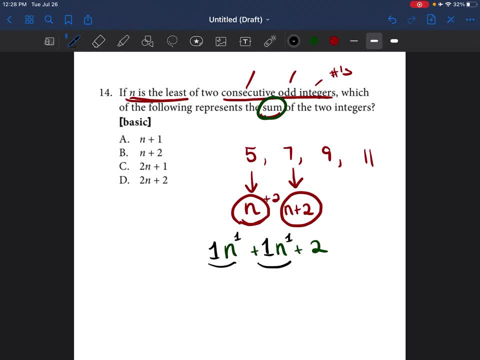 And they both have n to the same power, which is to the 1 power. So 1n plus 1n is 2n, And then we have the plus 2.. There are no other, just numbers by themselves, So we're just going to go ahead and bring down the 2.. 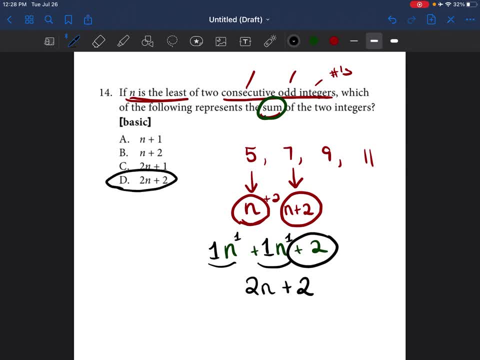 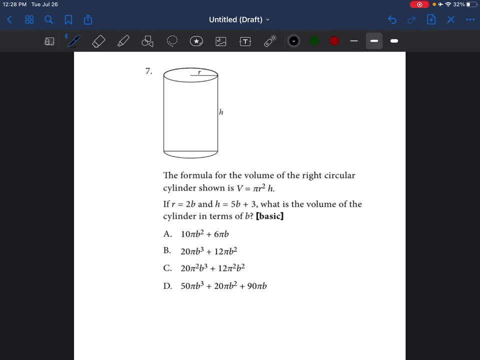 2n plus 2.. So the answer would be 2n plus 2.. So now we're going to go ahead and go to this next problem. It's asking us for the formula for the volume of this cylinder. is v equals pi r squared h. 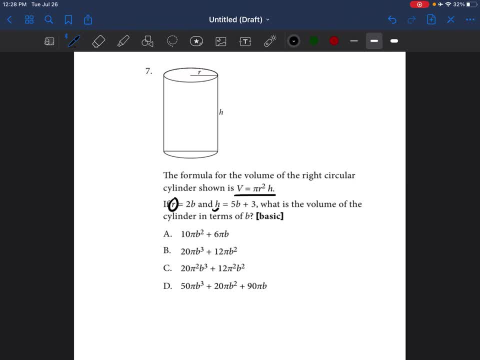 They're giving us what the value of r is and what the value of h is, And they want us to tell what is the volume of this cylinder in terms of v. So what they want us to do is they want us to just take this formula. 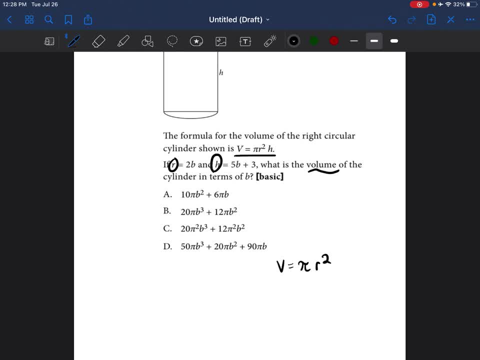 v equals pi r squared h, And they want us to fill in what the values are for r and for h. So before I go ahead and fill in what the variables mean, I'm just going to write it: pi times r squared times h. 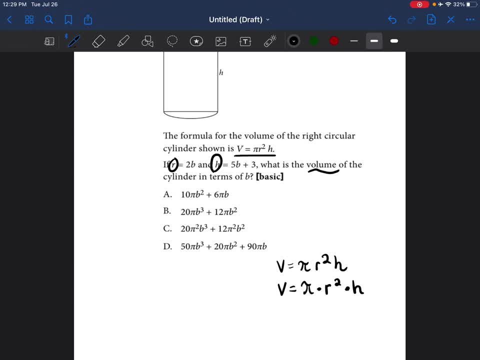 I'm separating them by multiplication signs. When they're written all together, they're being multiplied, So I'm literally just going to put the multiplication signs in between. Now that I have the multiplication signs in between, that's going to help me out. 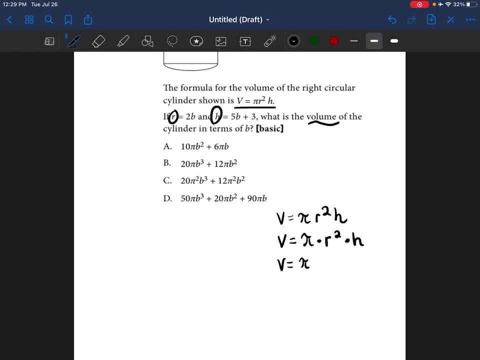 So now I'm just going to fill in what the values are. Pi just stays the same, but we know that r is equal to 2b, So instead of writing r, I'm going to write 2b squared multiplied by h. 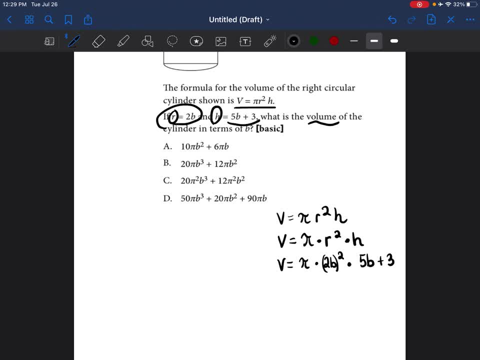 which is 5b plus 3,, 5b plus 3.. And I'm going to put that in parentheses. So now let's just go ahead and multiply things out. We're just going to bring down the pi, Then we're going to do 2b squared. 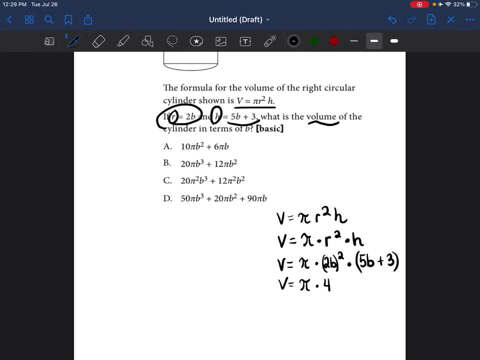 So 2 squared would be 4.. b squared would just be b squared. And then I'm going to go ahead and bring down the 5b plus 3.. And now I'm just going to multiply everything out. So now I'm going to do pi times 4b squared. 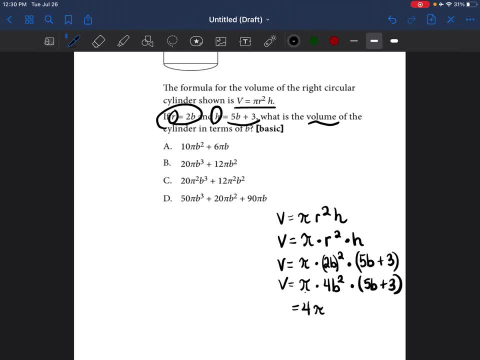 So it would just be equal to 4pi b squared. And then we're going to multiply that out by the binomial 5b, 5b plus 3.. So we're going to just distribute now. We're going to take this whole value and multiply it by 5b. 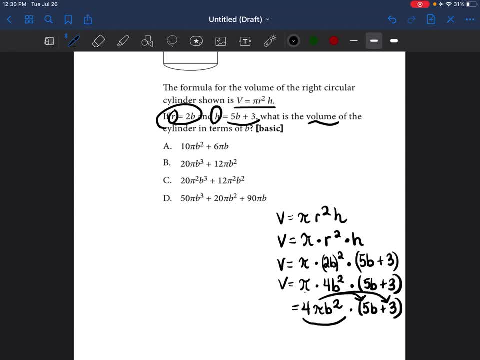 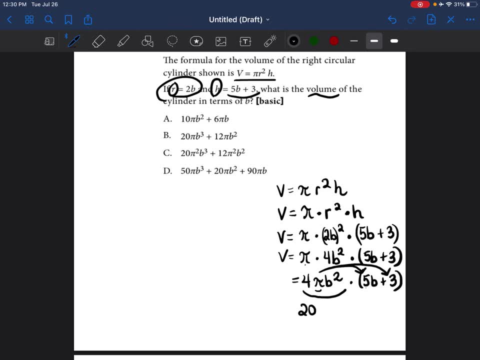 And we're going to take that whole value and then multiply it by 3.. So 4, we're going to multiply 4 times the 5, which is 20.. The pi: there's no other pi in here, So we're just going to bring down the pi. 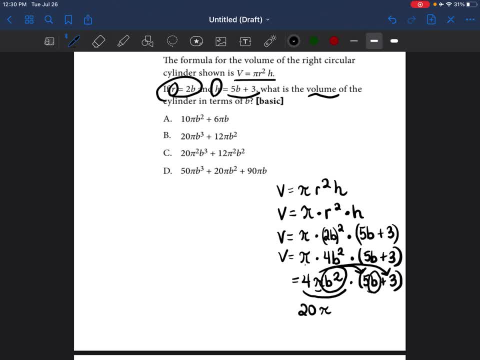 And then we're going to do b squared times b And I'm going to pull that over to the side. b squared times b, It's b to the first power. When you're multiplying variables that have different exponents, you just have the same variable and then you add the exponents. 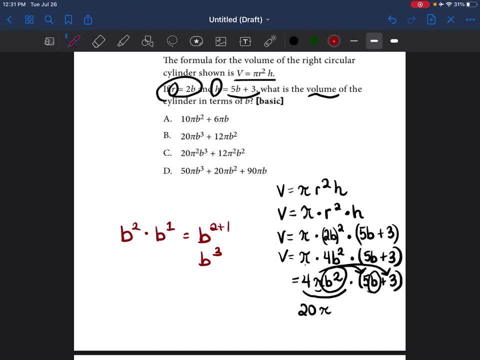 So it would be b to the third power, So 20pi b to the third power. So now that we multiplied everything by 5b, we're now going to multiply everything by 3.. So we're going to go ahead and do the same thing. 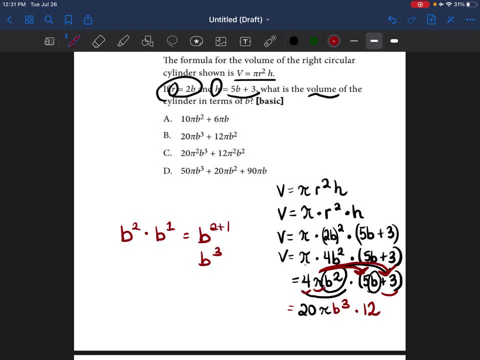 4 times 3 is 12.. There's nothing to multiply the pi again, So we bring down the pi. And then there's nothing to multiply the b? squared again, So we're just going to bring down the b? squared And our answer is going to be 20pi. b to the third power. 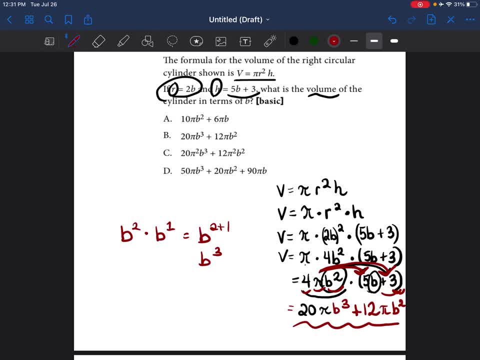 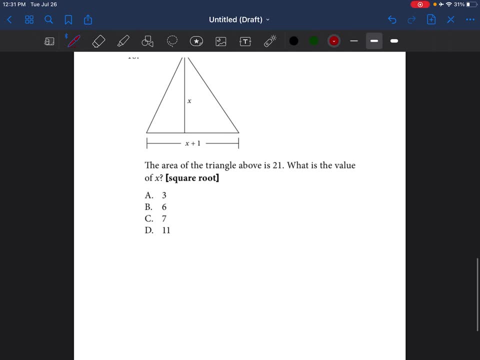 Sorry, this should be a plus sign Plus 12pi, b squared, And so we have this answer right there. So our answer would be b. So now let's go ahead and go to the third problem. So the third problem is: the area of the triangle above is 21.. 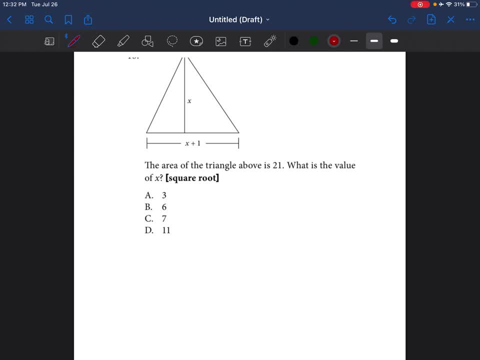 What is the value of x? They're asking us to take out outside information. If you're taking this test, you probably were going to give- they sometimes give you a sheet with all the formulas on it. If they do, that's wonderful. 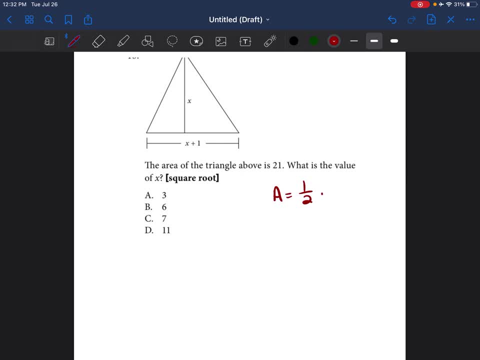 So the area of a triangle is area equals 1 half base times the height. So let's go ahead and put in what the base is. The base is the bottom of the triangle. So the bottom of the triangle is x plus 1.. 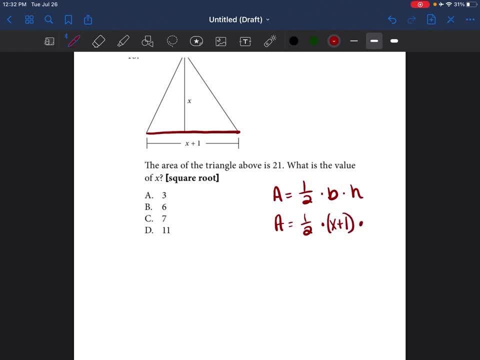 So 1 half times x plus 1.. And then the height is how tall the triangle is from the bottom, And so the height is just x. So you can do this the complicated way or you can do it the easy way. You don't have to be a mathematician in order to get this problem right. 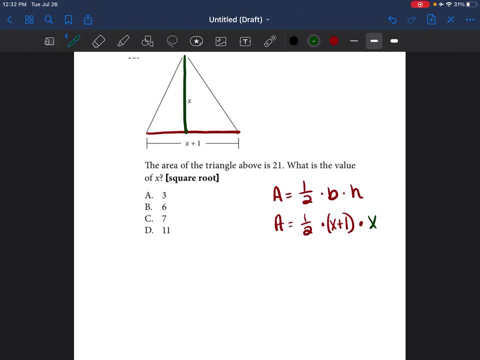 And so I'm going to do it the easy way. I'm going to show you the route that I would recommend taking so that you could just get the answer correct, And I'm just going to use my answer choices and I'm going to plug it in to see if I can plug in A, B, C and D. 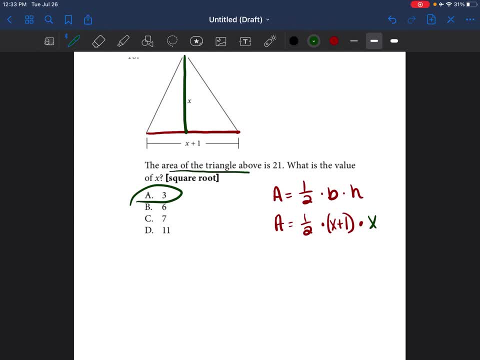 which one gives me the correct answer. So the area of the triangle is equal to 21.. So instead of writing A, I'm just going to write: 21 equals 1 half times x plus 1 times x, And first I'm going to use the number 3.. 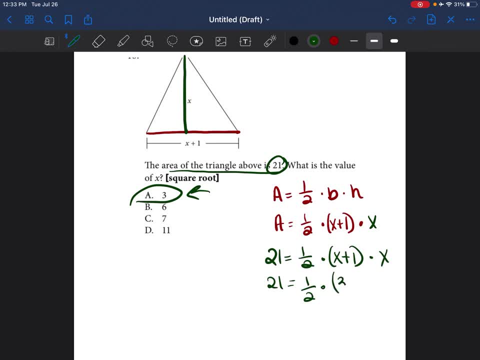 So 21 is equal to 21.. So 21 is equal to 1 half times 3 plus 1 times 3.. 3 times 1 is 4.. Okay, 1 half times 4 or 1 half of 4 is 2..